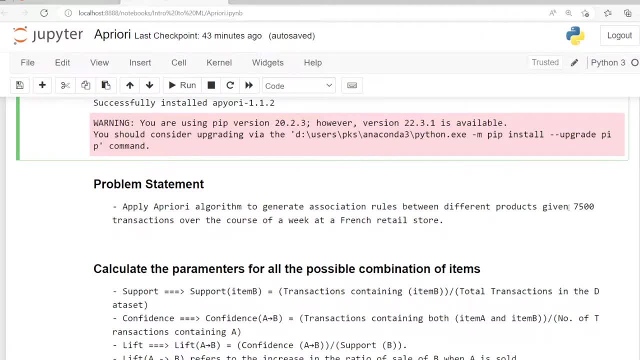 That means the data set is having 7500 samples. So in that 7500 samples different items are there. We have to identify when one item is buying by the customer what is the related item that customer is buying at the same time. 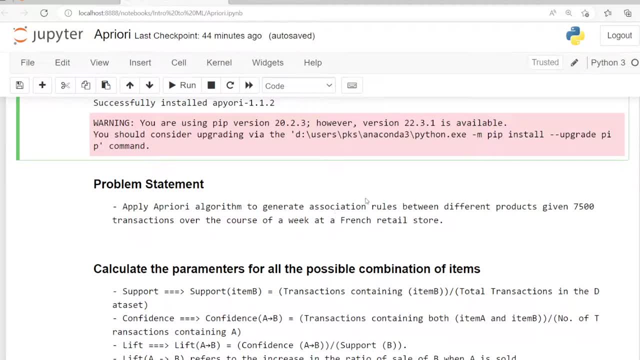 So if we are finding the association rule by accessing that sold items which are bought by the customer in the past in the same time, then we can arrange the products in the grocery store- Besides that, I mean near to each item to make the customer to buy easily and to access that items simply. 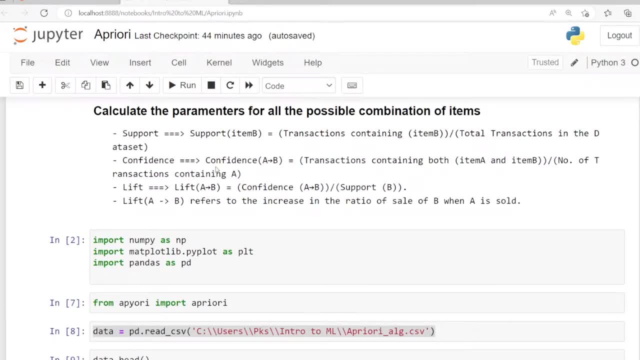 For that we have to calculate the parameters in Apriori Algorithm for all combination of items given in the data set. That means support of the item B equal to calculated by transaction containing. Also we have to provide the basis of the item B by calibrating the item A and sales. 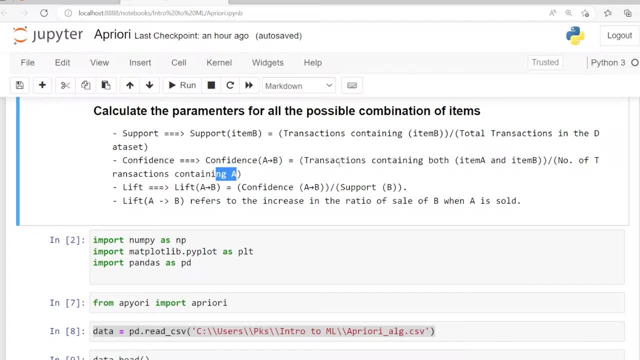 A plus B. As I said, the robot computer is always operating under the checking part and tracking the separate item set. As I said, the robot computer is always operating under the checking part and tracking the separate item set. So that means now we are assembly the item A and seemingly that Organisation Rightress is working well. Because that is also gotta have that reason. medical report, right, local information. but to factor numbers, which we are not used in our complexity, and really why the times when that МУЗЫКА an additional part of things that we are having, we have a dedicated addition to. 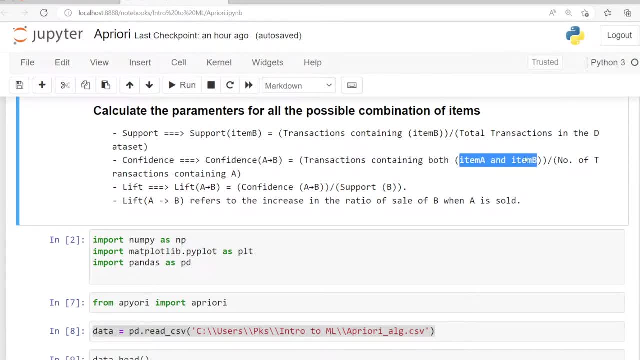 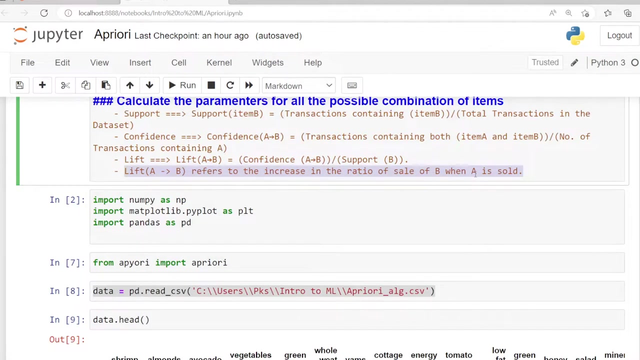 we should calculate for the both item a and b sold by the market at the same time. a lift in the sense lift refers how how much ratio we are increasing the sale of item b when the item a is sold. that means when customer a is customer buying the item a and how many times he is. 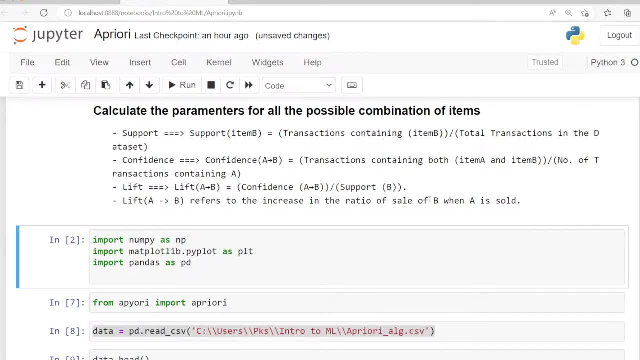 buying the b also. that is the meaning of this lift. so lift a implies b. that means whenever customer a is buying, i mean whenever customer buying the b product. all right, so that will be combined with the a. so that is calculated by using confidence of. a implies b divided by support of b. all right, so initially we are importing the numpy mat. 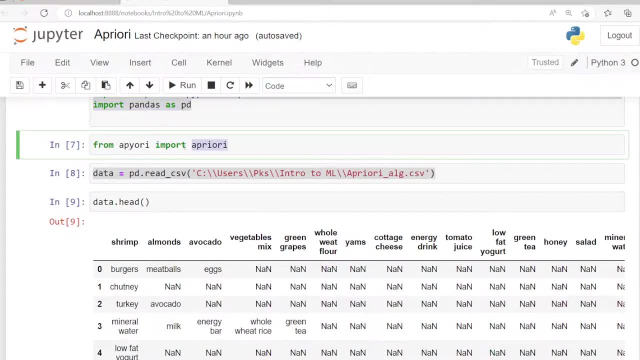 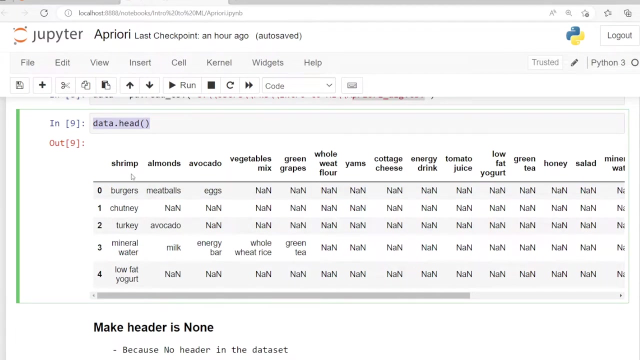 mat, mat, mat and the pandas package and we are importing the apriori algorithm into our jupiter notebook. then my file is available in this path. so i am accessing that path. then i am displaying the given data set using the pandas package. so here this data set is, displaying first five records. 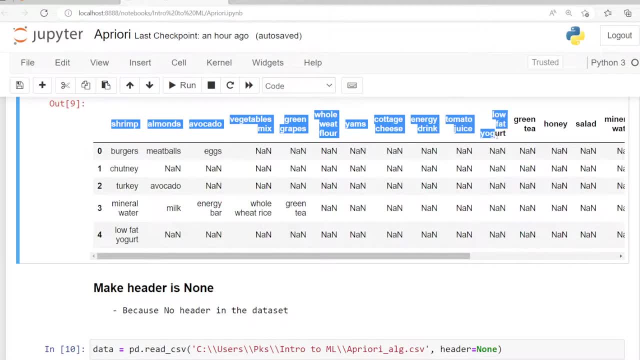 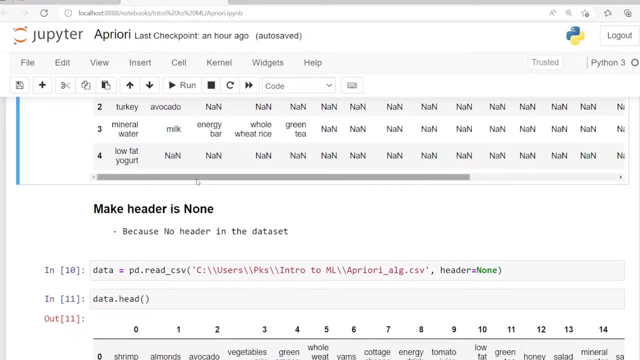 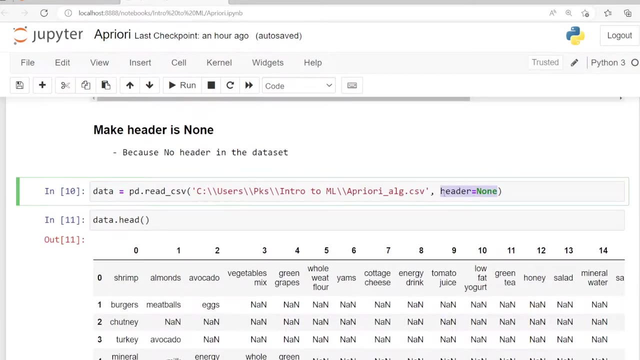 here. this data set is displaying first five records, but this is the header is not available in the given data set, so this is actually one of the sample. this is also one of the sample so we are making. the header is not available in the data set, so we are removing. we are accessing the file without header, so here. so this also is one of the. 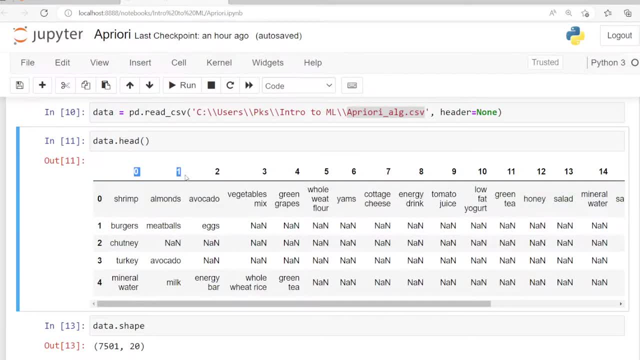 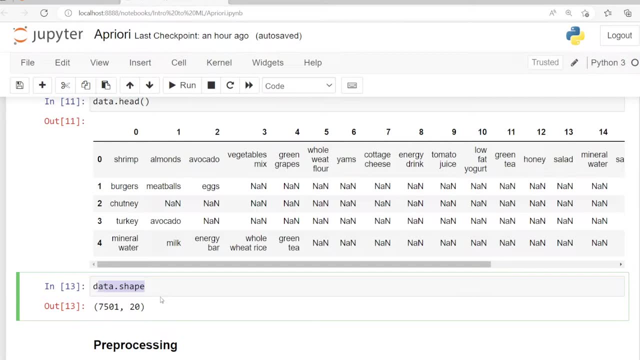 sample in the given data set. so here a default header is given as a zero to seven. because now we have some data sets. we are saying to the data set we are creating a new one here, so we are feature first feature like that. so here I am displaying the step of the given. 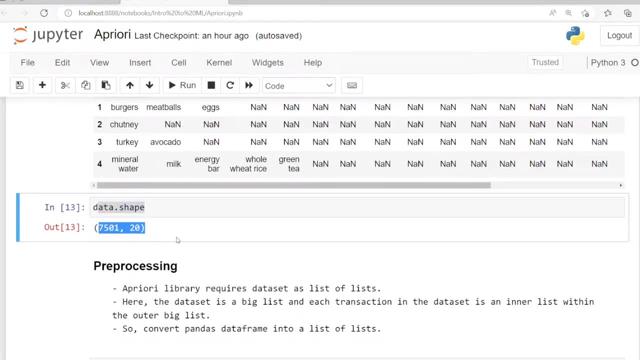 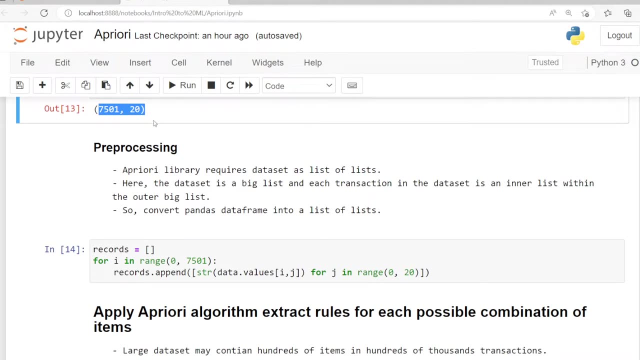 data set 7501, comma 20. 20 is the number of features, then we should apply the pre-processing here. actually, here we are having the data set in the name of set of columns. under set of I mean a number of rows. number of columns under number: 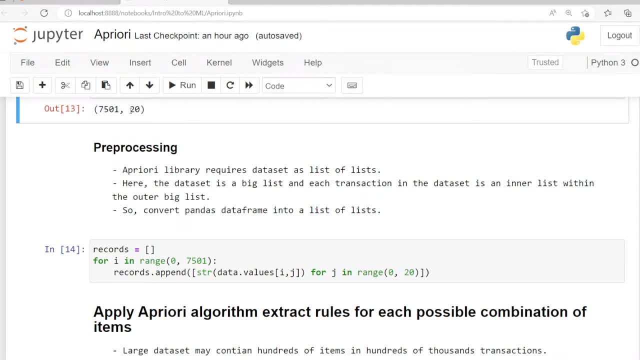 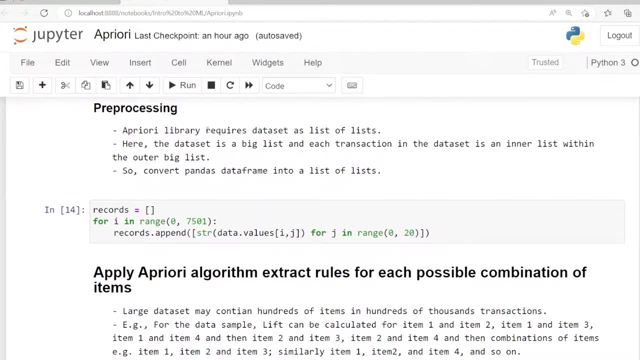 of rows. so this can this: this should be make as a number of transactions for a prairie algorithm. so for that making transactions, we need to convert that data set into a list of lists. each list will contain transaction. each list will contain transaction that will be formed in the in the procedure procedure list. 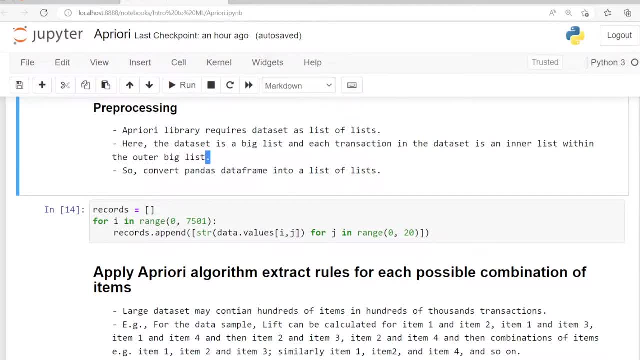 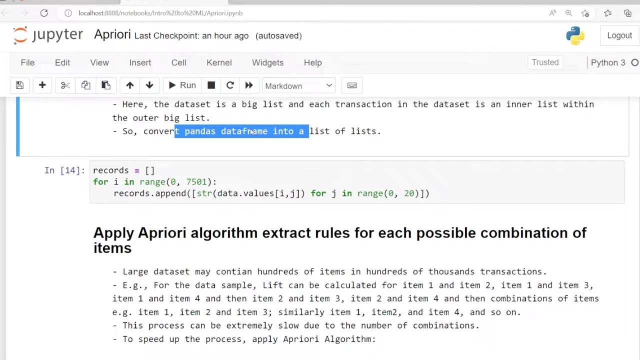 which is having the inner, the inner list within the outer big list. the entire data set is called outer big list. then each transaction will be inner list into the outer big listed. so this can be converted by using the data frame upon. does that I mean converted by from the? 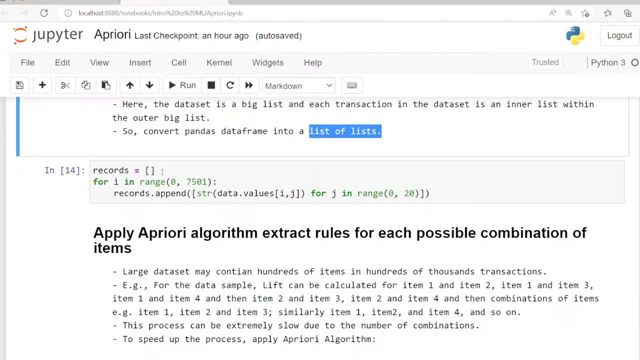 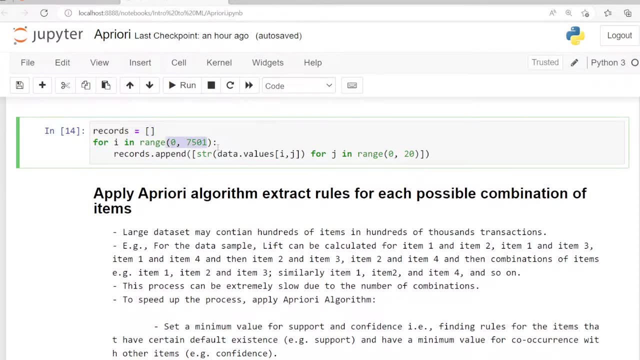 pandas data frame into list of lists by using the for loop. here I am making empty list. name is records. then I am moving from 0 to 7501 rows year. then the data set is having 7500 samples, the it is. so we are making the. 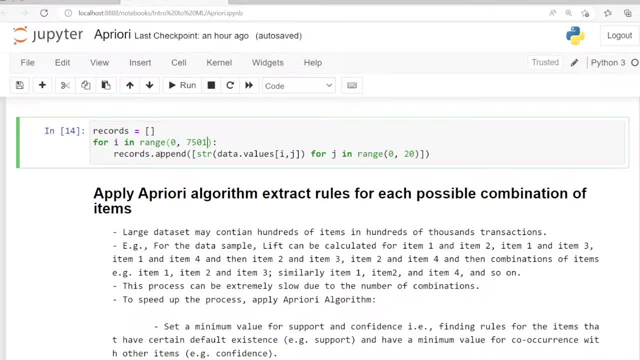 7,500 to 1. we are creating the records by using the values of the data, that is, the data set. so, based upon that, we are keep on creating the list. we are keep on creating the records, not a list. we are keep on creating the records. so, as I said, 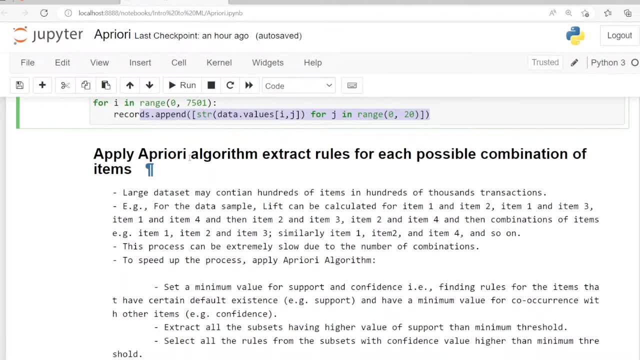 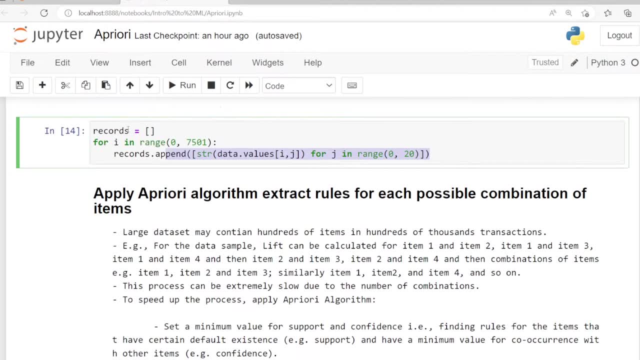 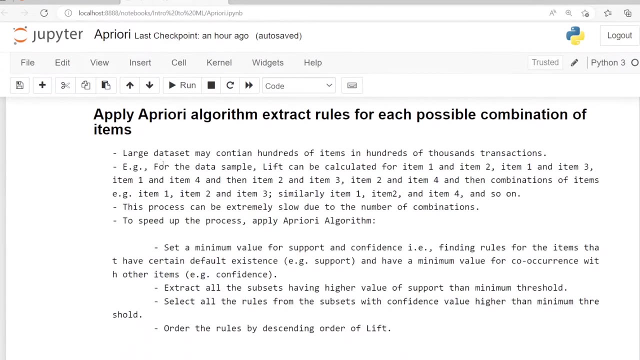 okay, then here we are, applying the apiary algorithm to extract the rules. so here the list is created in the form of records, in the variable of records. so here list is created by using the variable records it is stored, applying the apiary algorithm to extract the. 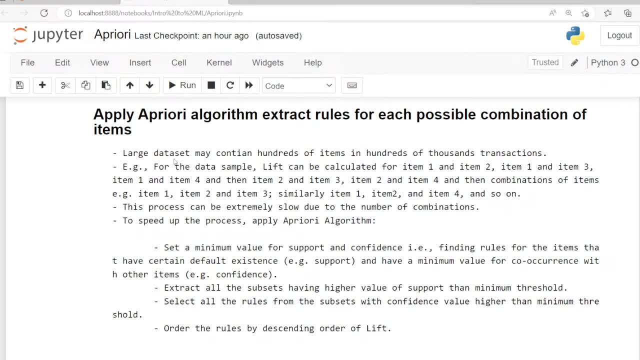 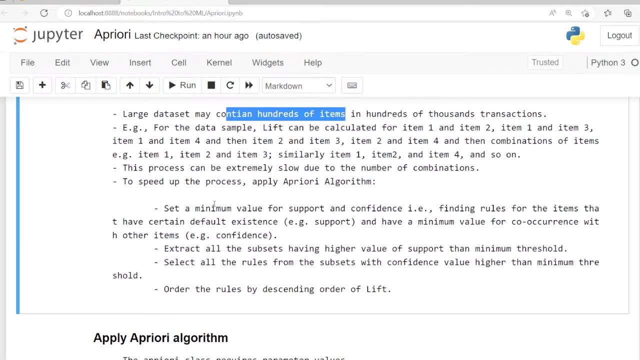 rules for each possible combination of items. here the large data set is having the seven thousand five hundred transactions. for that we have to identify frequent item sets. frequent item sets will be calculated by using the minimum support count and confidence. that means which is finding the we are. we are interested to find the rules with the different 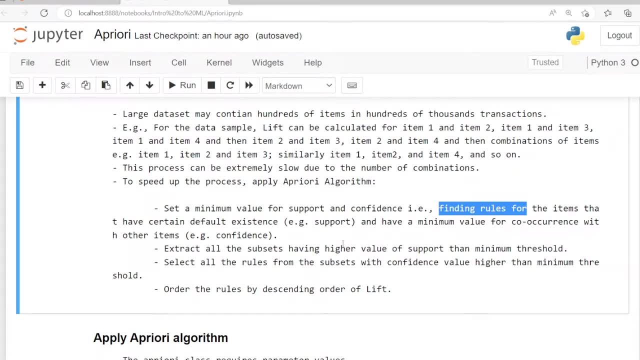 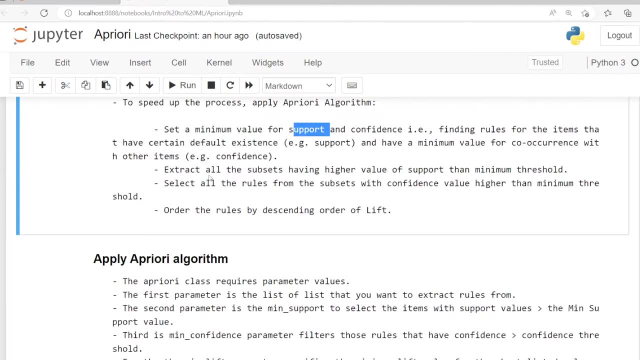 combination of the items to sell to the customer so that should be satisfy the minimum support and minimum confidence. so here we will extract all the subsets whichever record is having, i mean whichever item is having more than the minimum support count and minimum confidence. so we will use that then, based upon 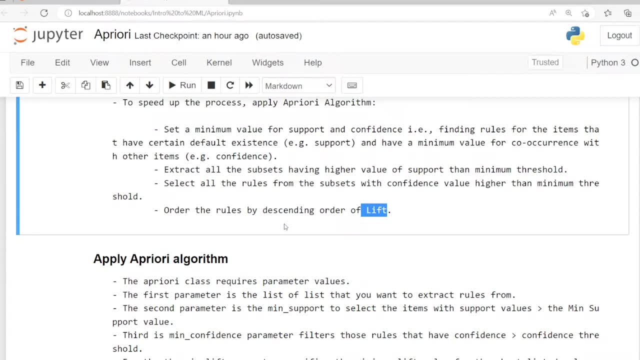 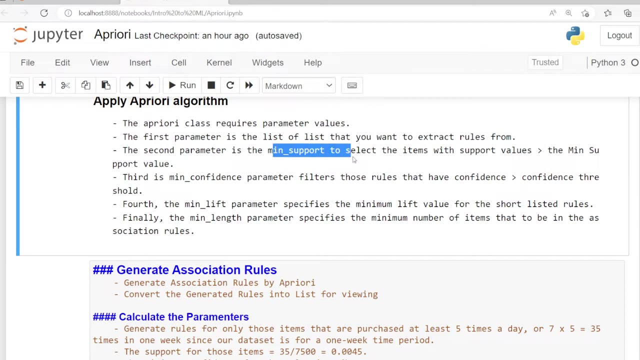 the minimum support count and minimum confidence we will sell the- i mean the customer buy that products in the different combination. so for that we will calculate the first extract, the rules and based upon the minimum support count and confidence we will use the minimum lift parameter to match. 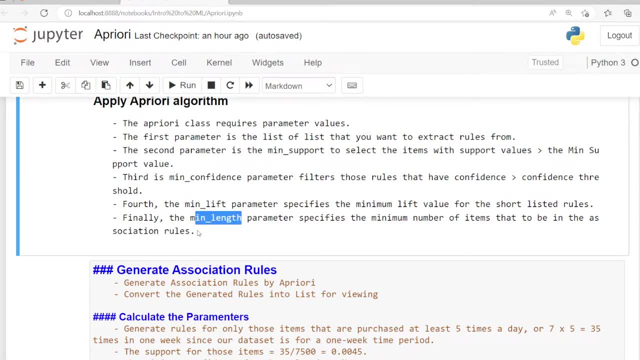 that combination. finally, the length of the combination. also we have to use minimum items. that means each, each. whenever the customer is buying, at least he will take one more product from the market. so minimum two, two items combination we can fix by using the minimum length parameter. so here we are. 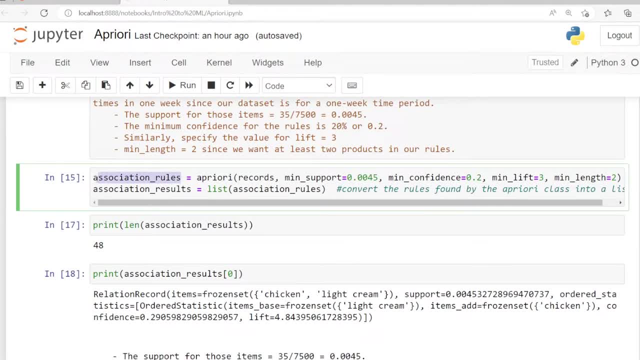 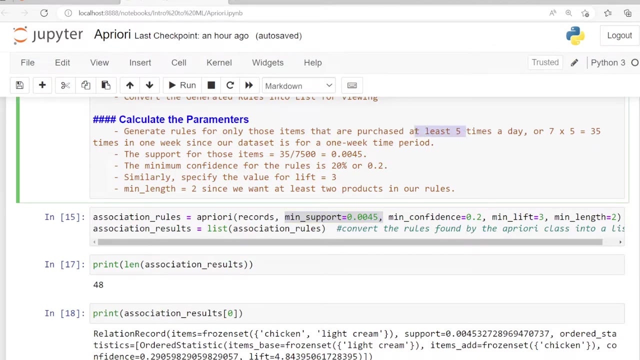 creating the rules of by using the apriori algorithm. records are 7500. minimum support count we are calculating here. we are calculating for the minimum support count based upon each product is by at least 5 times by the customer in seven days. so the whatever product is sold 5 times that. 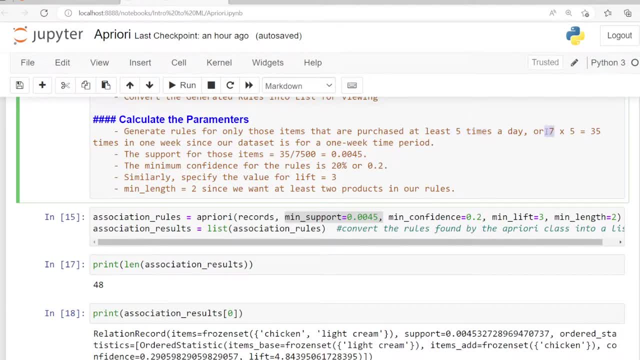 will be considered in the data set for 7 days. so 35 times it will be appear minimum in the data set. okay, so 5 times it is sold throughout the entire week, 7 days. so thirty five is the minimum support count we are using. so 35 number 35 times it is appearing in the data set out of seven days. when we are sending the platform for the. 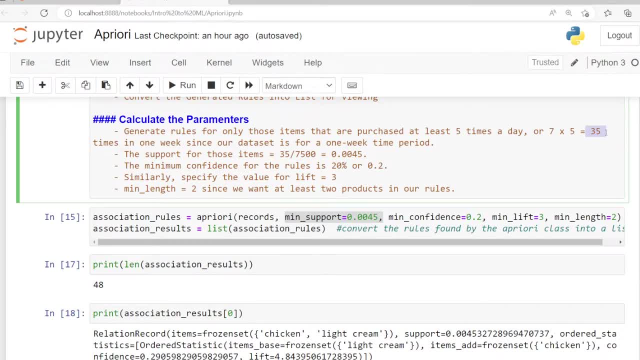 five times and minimum support count based upon the minimum last din Instagram sleepnumber times. we are using, so 35 times it is appearing, starting from here. we are using, so we are using manages من find that we want ما the data set out of 7500, so we are getting. the minimum support count is 0.0045 minimum. 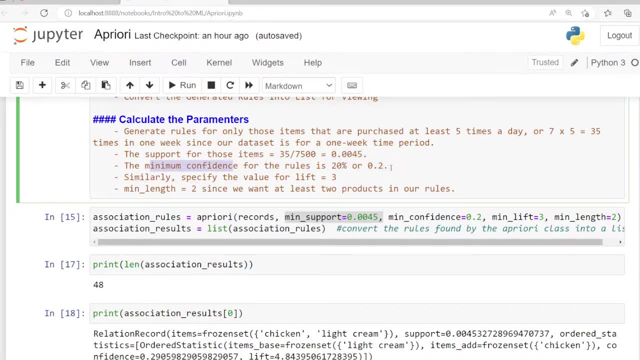 confidence we can set manually by. so here 20 percentage of the minimum confidence. so we are setting 0.2 here and lift minimum. lift is here 3, 3, 3 products: yes, set set here so the length of the items to set the rules, to create the rules we are using, minimum at. 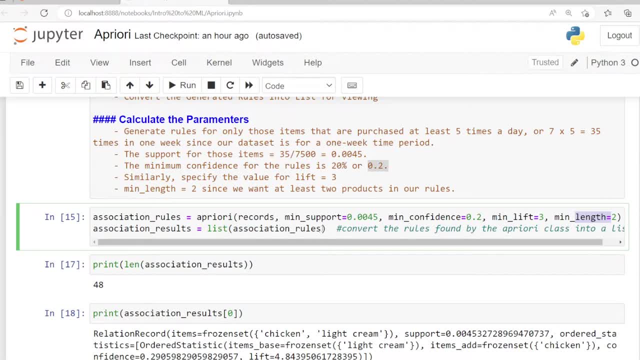 least two items to generate the rules. then, based upon the apriori algorithm, with these arguments generating the rules, this rules cannot be viewed by directly so that rules are assigned into. I mean the rules are created in the form of list. so we are applying the list method. 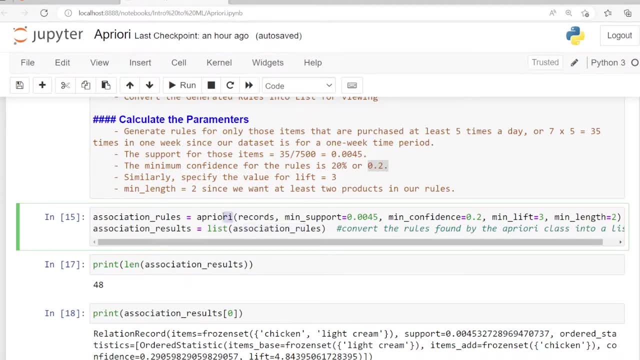 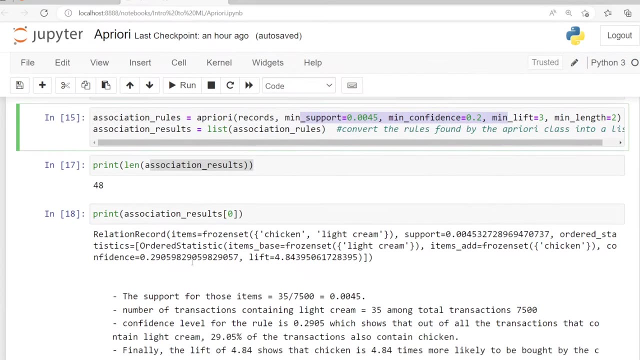 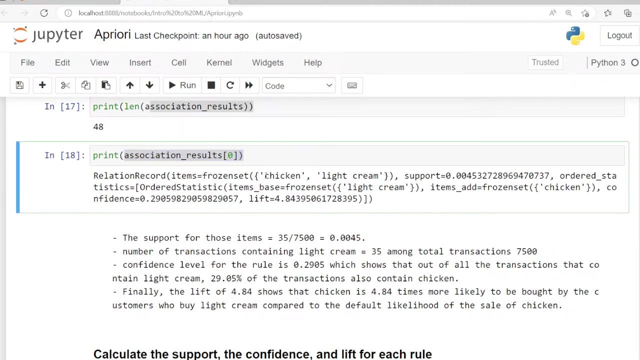 To convert that output of this apriori algorithm into list of rules, list of rules. so association rules are generated here in the form of list. 48 rules are generated based upon this minimum support count and confidence. here we are displaying the first rule. the first rule is having a 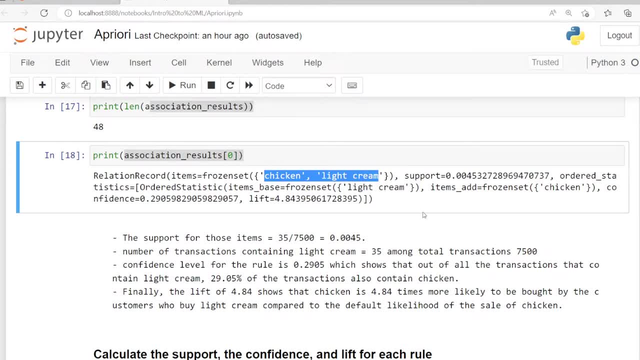 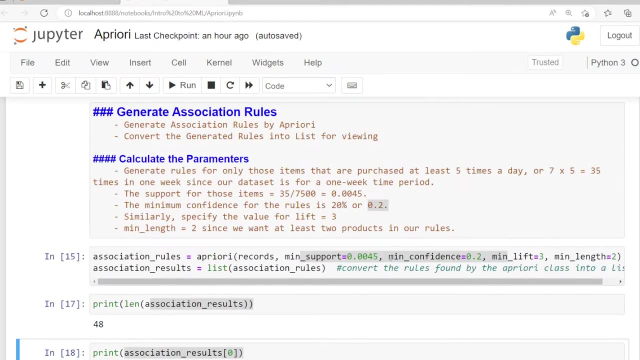 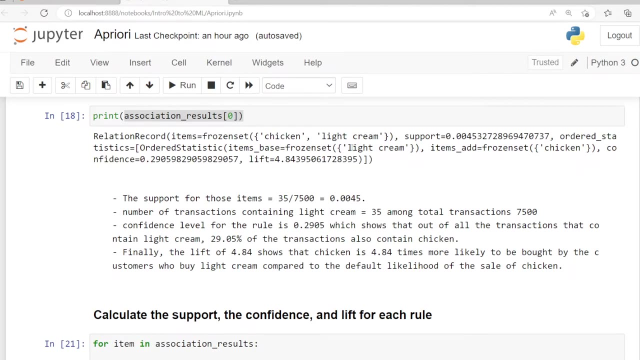 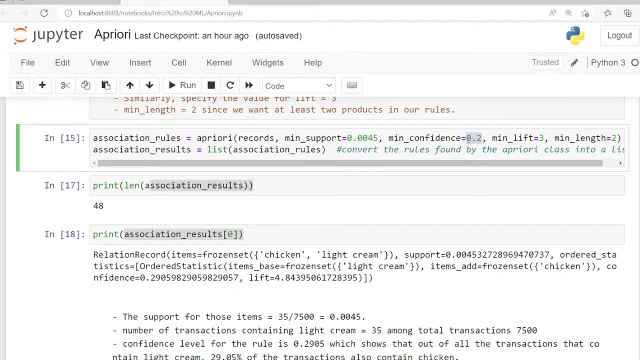 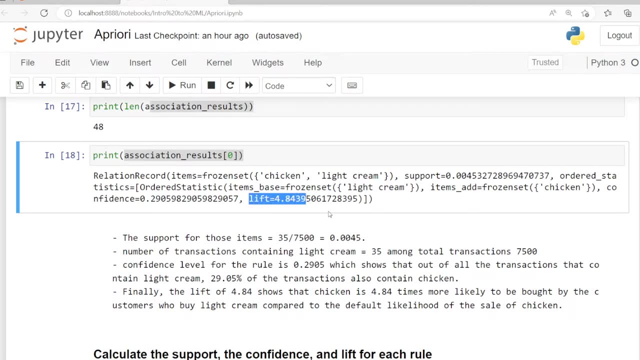 given 0.29. here we have given only one digit, so it is taking a number of digits. so here lift what is the ratio of by buying these two products combination. so 4.84. so that is what given here. so 4.84 times more likely to buy by the customers who are buying the light cream. 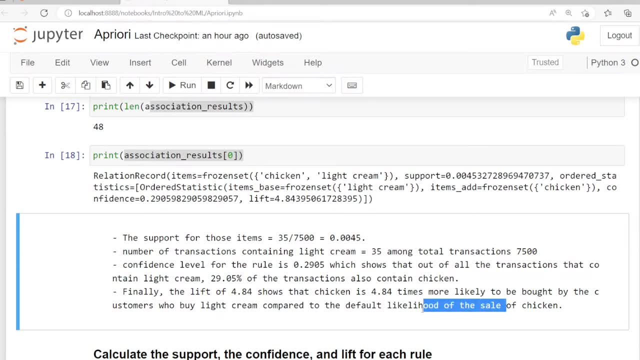 compared to default likelihood of sales. so that's the possibility of 4.84 times they are buying. whenever they are buying the chicken, they will buy the light cream. so that's the possibility of 4.84 times they are buying. whenever they are buying light cream, they will buy the light cream right in the combination. so 4.84 times they bought in. 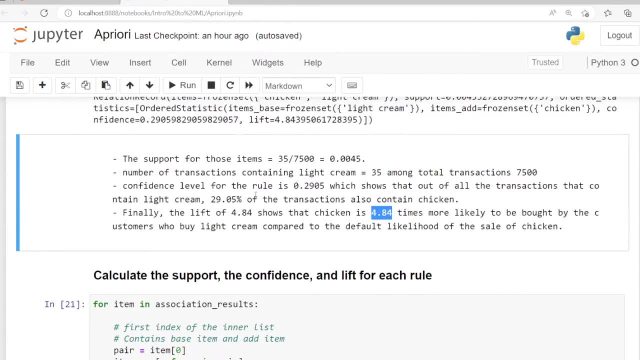 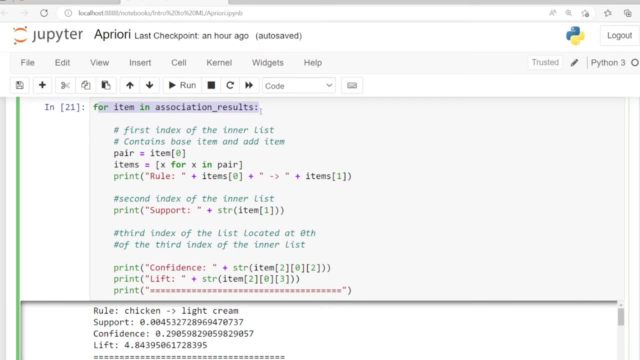 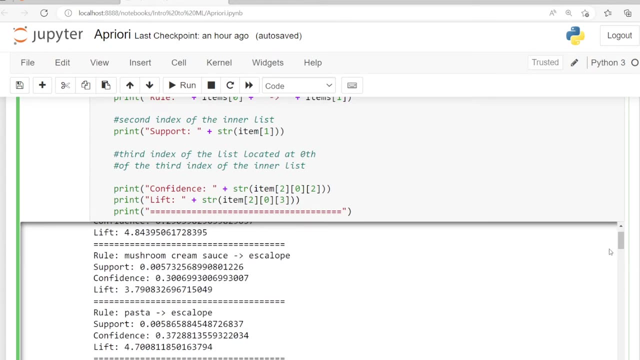 a week. so that's what given here. so this is for only single rule. then here we are creating the association or results. i mean rules for inner list, different combination here so many rules are there, so totally 48 rules. actually totally 48 rules are there. so among the 48,